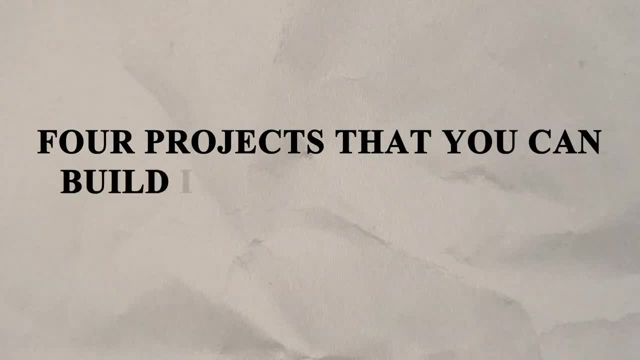 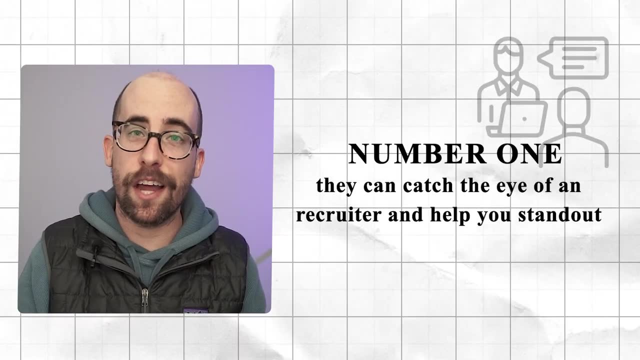 Okay, so today we're talking about four projects that you can build in a week that will get you hired. Projects may be the single best way to help you get a job, because- number one- they can catch the eye of an interviewer or a recruiter and help you stand out And they prove that you have the 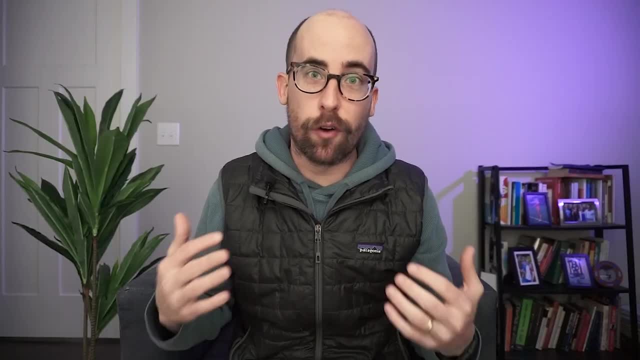 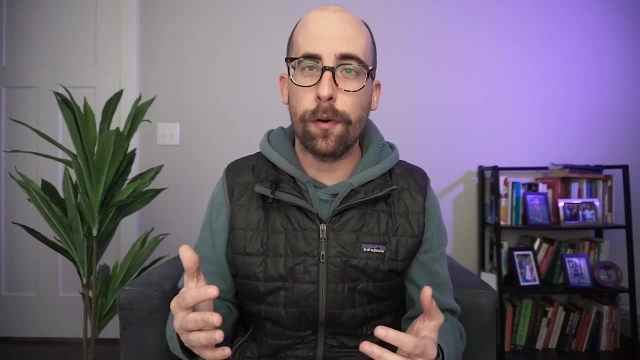 skills to do the job that you're applying for. If you do it right, it's a great way to stand out. But the question I hear so often from either junior developers or even mid-career developers or people just looking to get into the industry, is: what do I build? So for that reason, I'm going 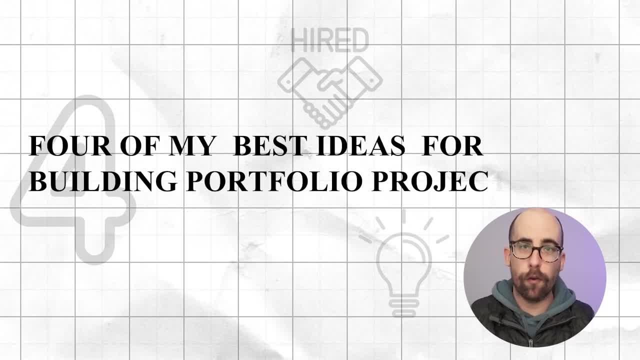 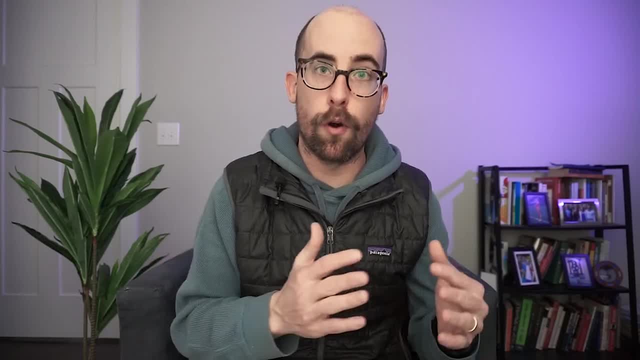 to take you through four of my best ideas for building portfolio projects that will get you hired. A quick note before we jump in. I'm assuming these are full stack projects, but depending on whether you're more front end or back end oriented, you can adapt these kind of to fit. 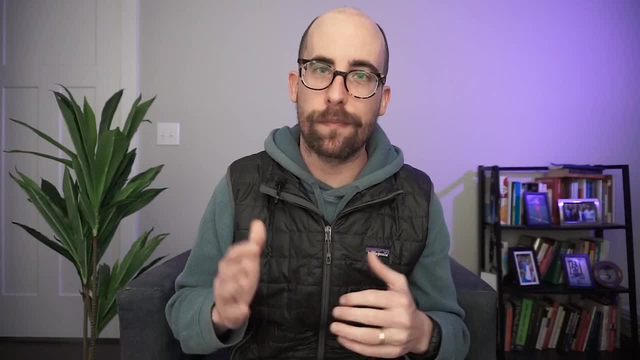 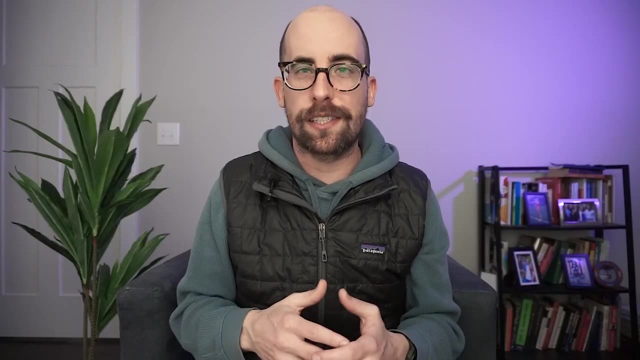 your needs and fill in whatever gaps you might have. So let's go ahead and get into it. Okay, the first project is building a landing page for a company, And I know I just said that the project can be front end or back end oriented, depending on your preference. This doesn't really fit the 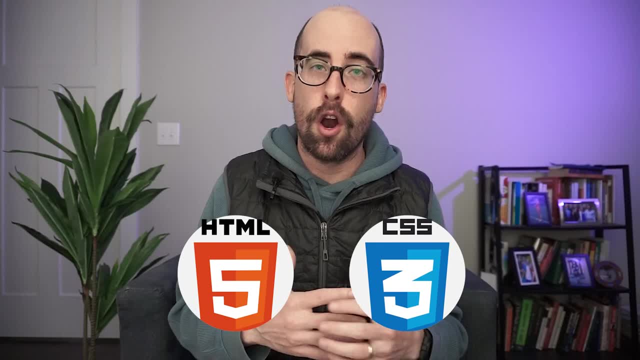 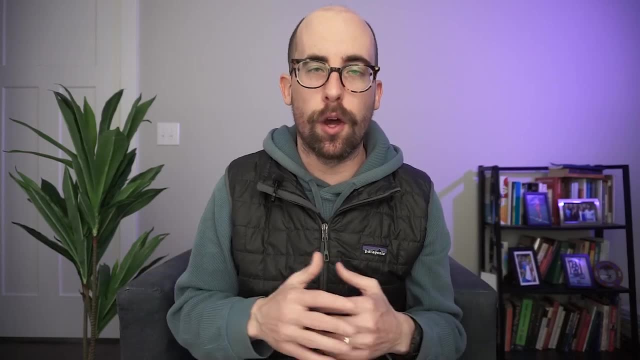 bill, And the reason is, I think, that HTML and CSS are core skills that everybody should be at least competent in, regardless of whether you're more front end or back end oriented, So this will be good for everybody to do. I think there are a few reasons that this is a good project. Number one: 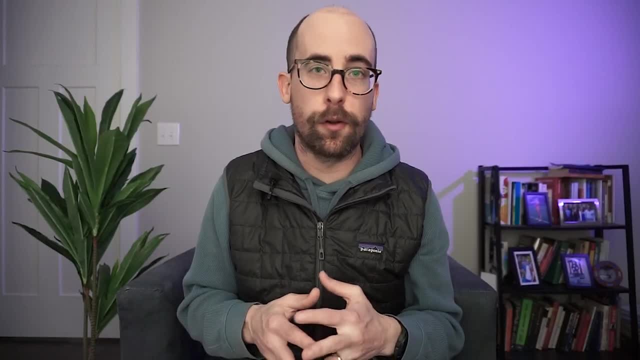 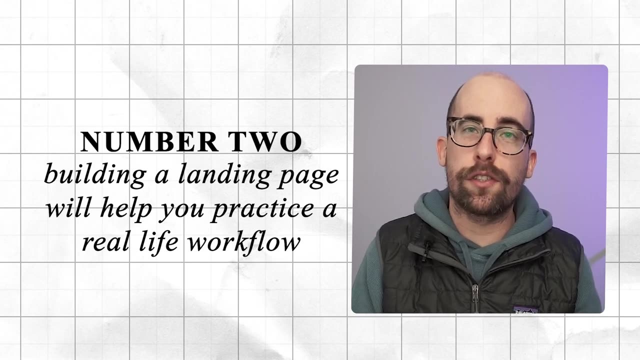 companies need landing pages. So, assuming you have these skills, you could go get freelance work or slot in at a company and immediately provide value. So that's pretty cool, And building a landing page will also help you practice a real life workflow, So as a front end developer. 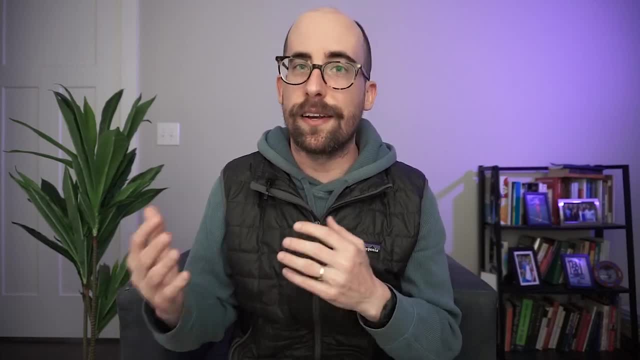 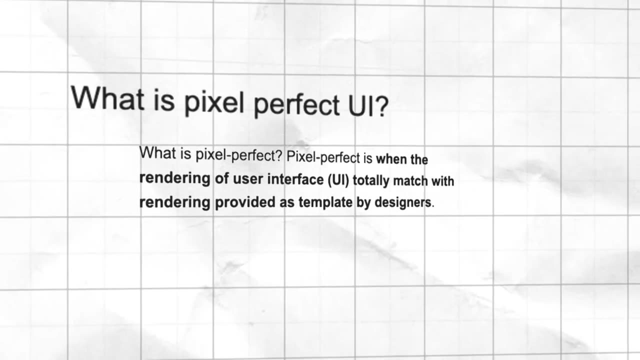 or as a full stack developer. a lot of times you're given a design, either in Photoshop or Sketch or Figma, And you have to implement that in a pixel perfect way. Pixel perfect is just. it matches the designs exactly. So if you do this project, then you will have mastered that real 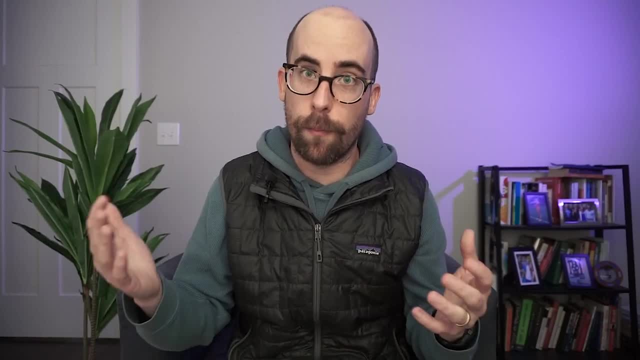 life workflow, And it'll be helpful when you actually start doing it on the job. And so, assuming you've bought what I've said so far, you may be asking yourself: well, where do I go to get designs and projects? And I'll tell you, you're going to have to do a lot of work And 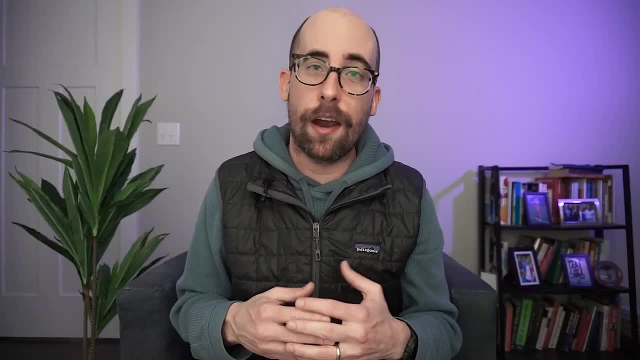 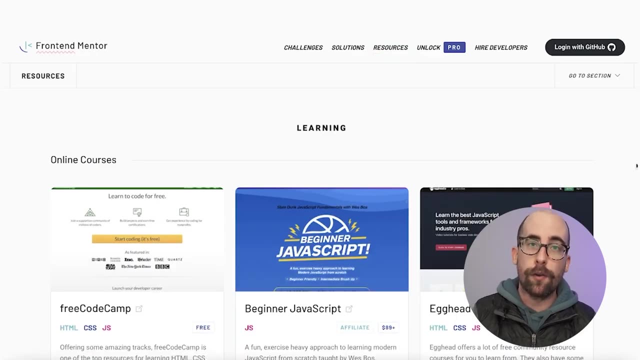 practice this real life workflow, And I'm going to tell you about a website that I mentioned before on the channel, And that is frontendmentorio, And the purpose of frontendmentorio is basically to do what I'm talking about. You get designs and then you implement them, And so it. 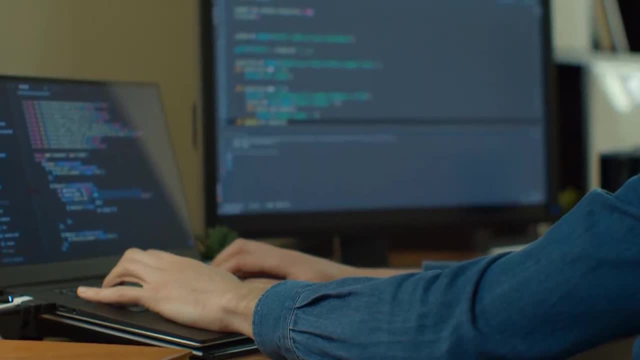 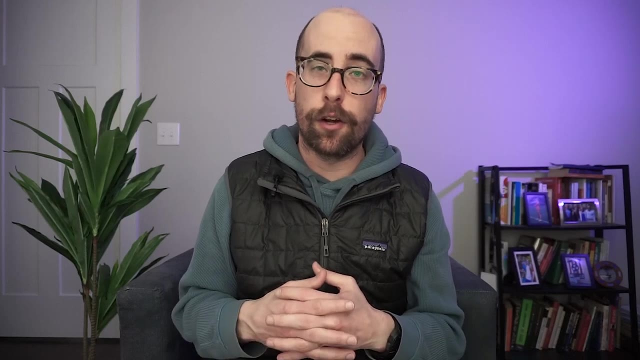 teaches you that real life workflow is a great opportunity to master your HTML and CSS and maybe even a bit of JavaScript And, like I said, you can make this more front end or back end oriented. So let's say you're a more back end oriented person. You can build an API to receive form submissions. 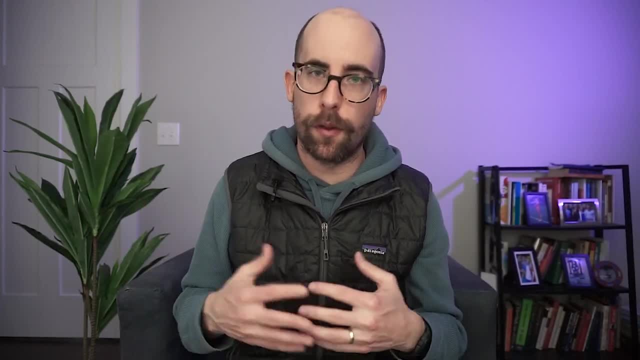 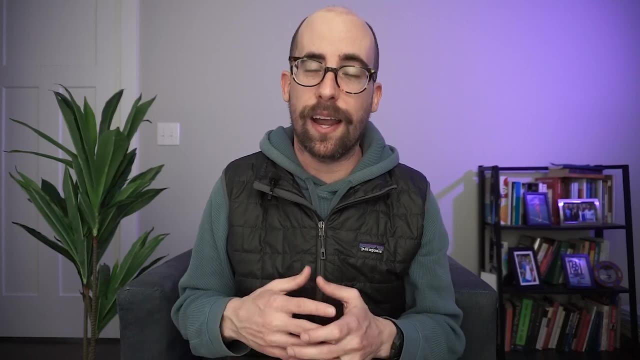 and anything you could think of Really. you can build in automations, you could build in scraping, you could kind of do whatever you want, And so I think this is a great project to get started. Like I said, you could build it within the week and you could have a really nice looking. 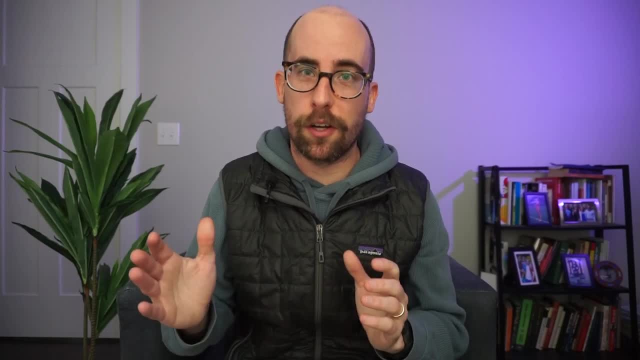 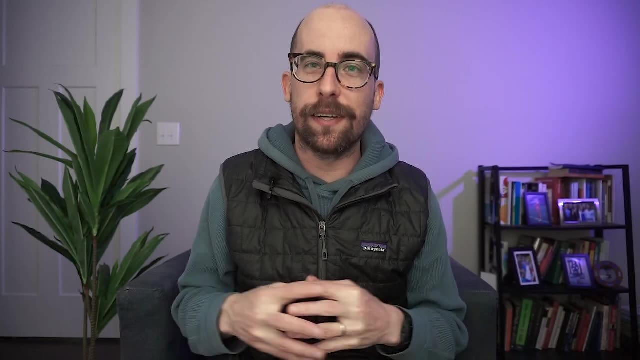 portfolio piece for you. With that said, let's go on to the next project. Okay, the idea for the second project is a game, And I think maybe a few months ago people would have dismissed this, But since the popularity of Wordle, I think people are way more into games and thinking about how. 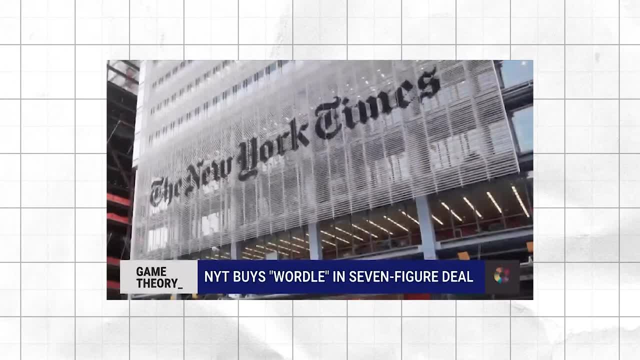 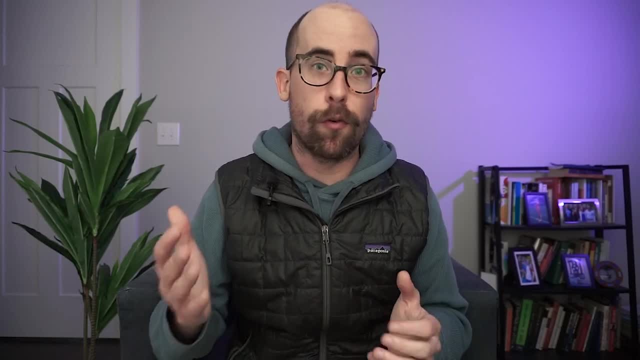 can I build a game that people are really into, Especially since Wordle sold for several million dollars to the New York Times? It's on people's minds right now. But even disregarding Wordle, I think a game is a great portfolio piece. There's a. 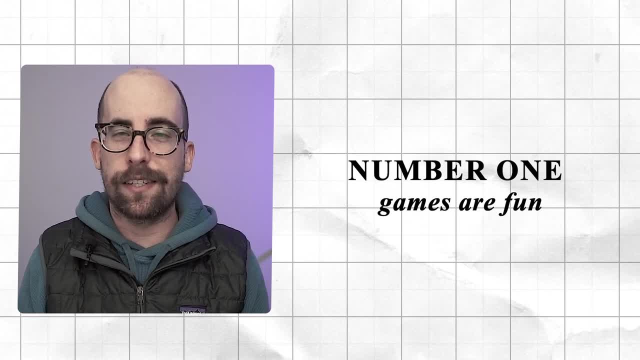 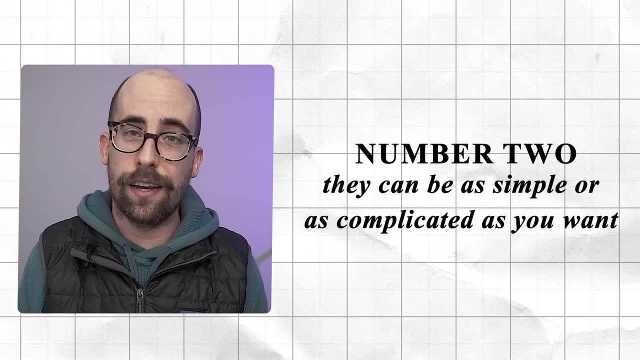 few reasons for that. Number one: games are fun, And so I think it's a good way to get whoever is reviewing your portfolio engaged in the project. Number two: they can be as simple or as complicated as you want, So you could do a simple text based game, kind of like the game in the movie Big 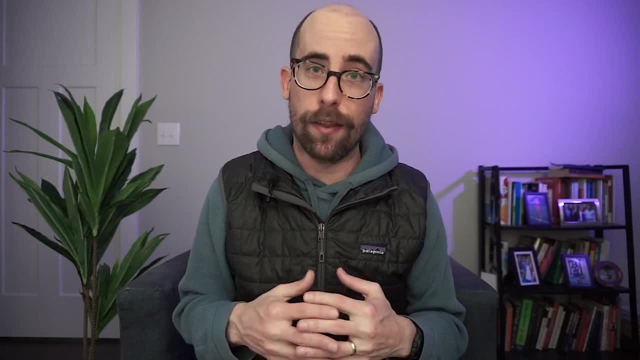 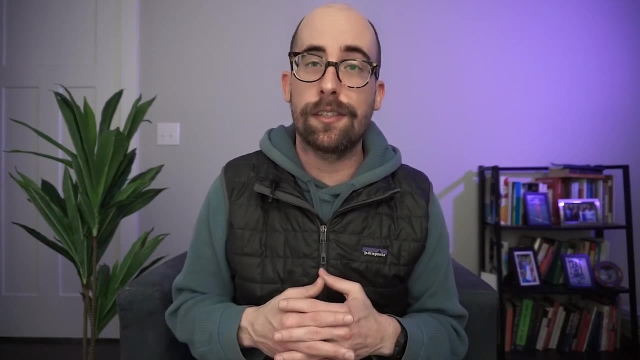 where you're simply entering commands, Or you can make it complicated like something like Wordle- even though Wordle is not that complicated- or like a pong or something that has a lot of interaction, something that has web sockets. you can really go crazy on this And you can make it. 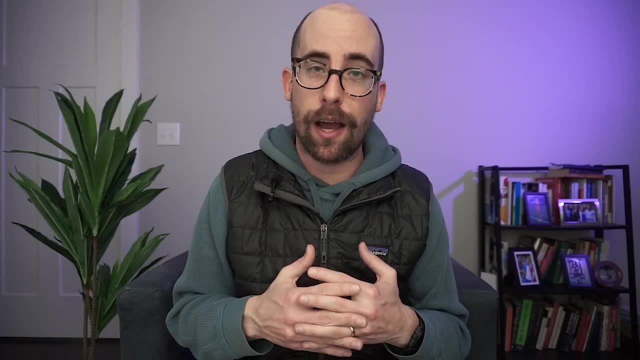 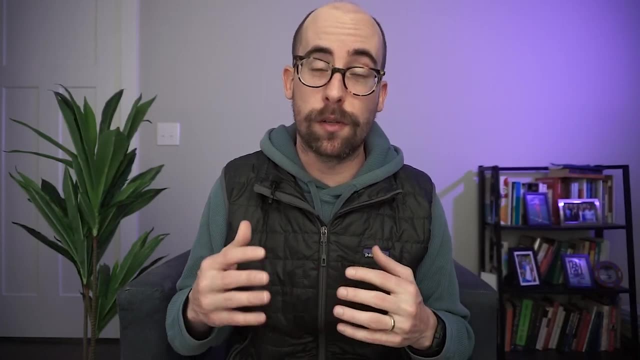 as complicated as you want from a back end perspective. So I mentioned you can kind of spice these up. you could do user authentication and leaderboard, which is something that Wordle didn't have because the creator was focused on not having a back end. But the good thing is when you're. 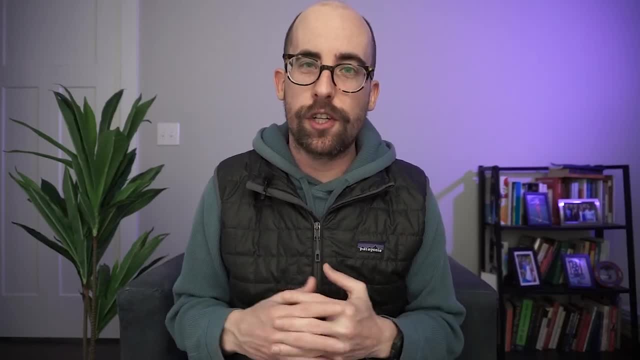 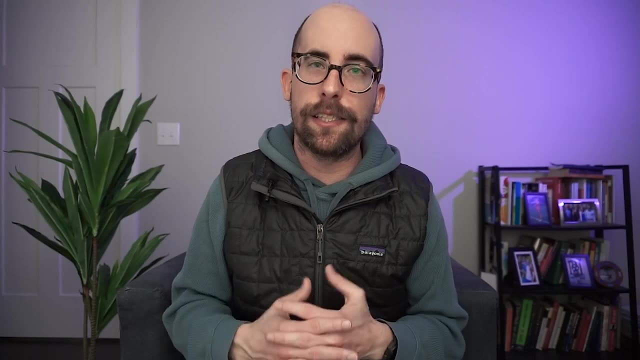 making your own game. you can do whatever you want And, depending on which direction you take your game, it could teach you some really interesting skills. So there's no need to learn C++ or Unity or anything crazy for this. You can make a game using HTML5 canvas and have a lot of fun And depending 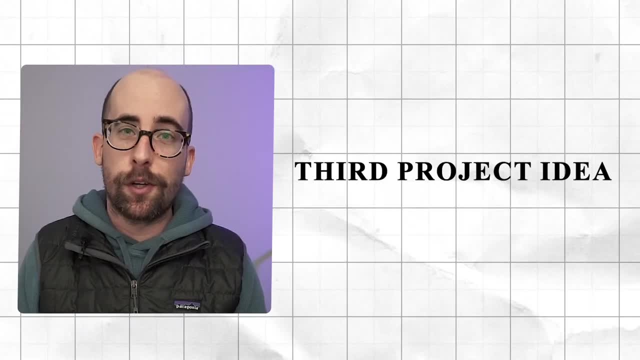 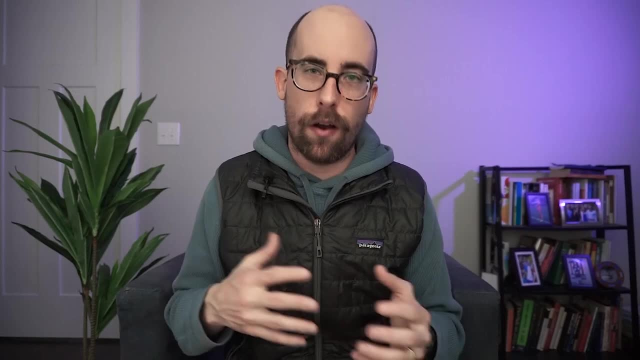 on what direction you go. there's a lot you're going to learn. And that brings us to our third project, which is a database. And I put database in quotes because it is data, but there's also a front end around it, So let me explain what I mean. I think looking at a good example of this is 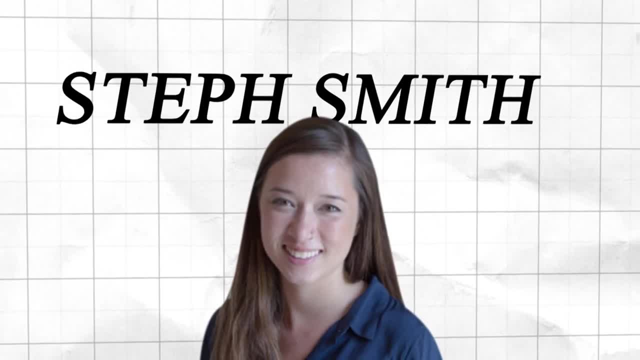 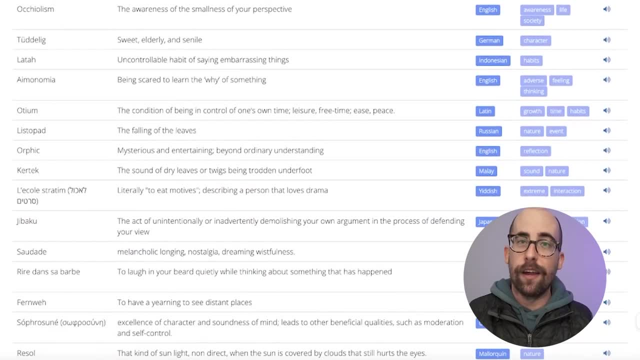 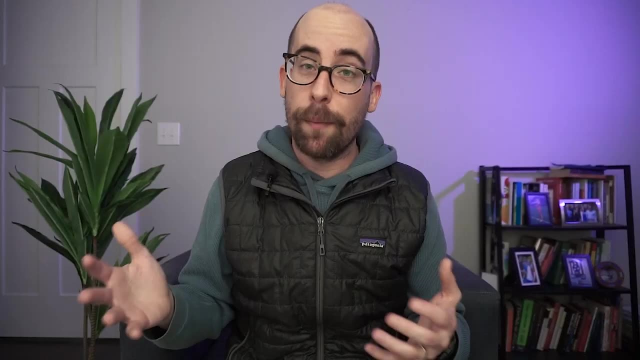 probably easier than me explaining. So I'm thinking about this project from Steph Smith called Younoya, which is basically a database that she has around words that are really hard to translate into other languages. They kind of only have a meeting within their language, And so this is basically just a list, a table with columns where you can look at. 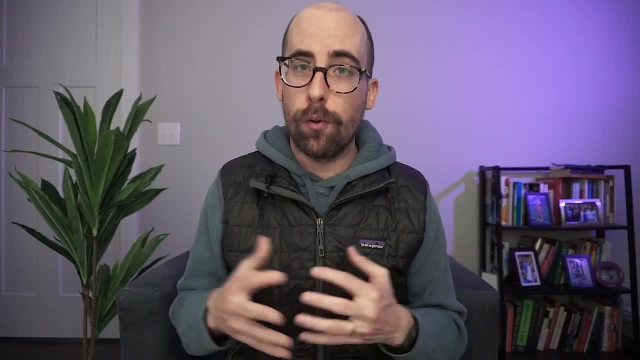 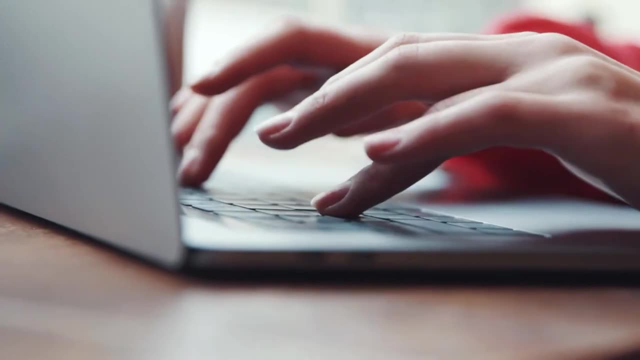 things. you can sort search filter And that is pretty cool. It makes a great project idea, Number one because people like data And number two because there's a lot of directions you can take this. So, for example, you can select the data on your own and you can simply have it on a front end in JSON. 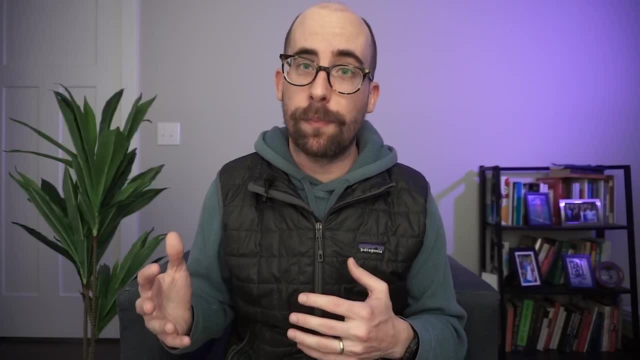 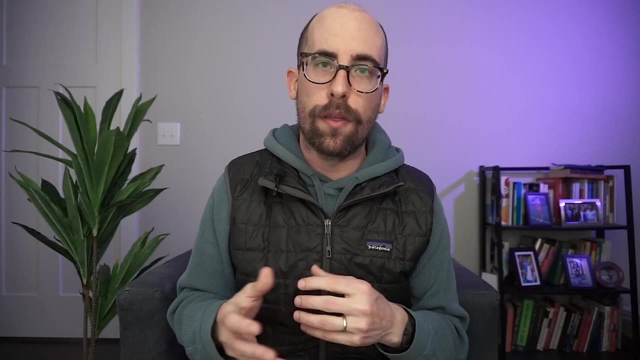 or you could have a real API where they're actually requests being made to a back end. You can make it a full stack node app- which I'm pretty sure Steph Smith did in this particular one- where the front end is just a template and it's mostly back end- kind of business logic- And you can do a ton of other things to actually get the data. So let's say there are data sources that you're interested in, You can write a scraper that goes out on a cron job night at midnight or something and collects and updates your database. So you can really take. 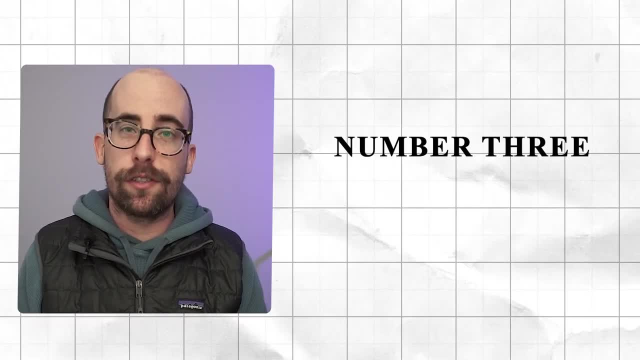 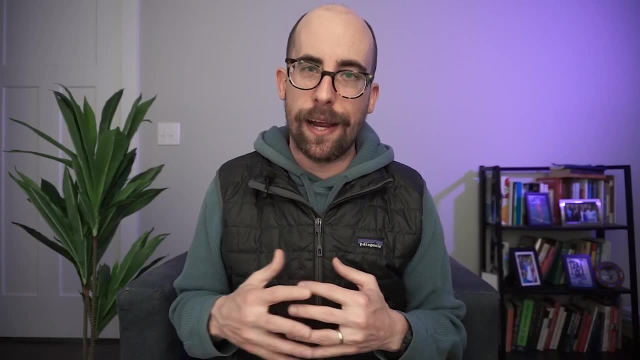 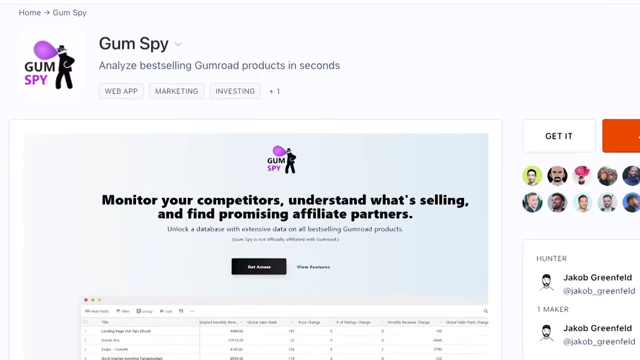 this in some pretty interesting directions. Another reason this is interesting is that people are willing to pay for data. So I'm particularly thinking about this guy, Jacob, right now, who has a bunch of data-based products that he collected by scraping, basically. So he has this thing called gum spy, which is basically data on what's selling on gum road. 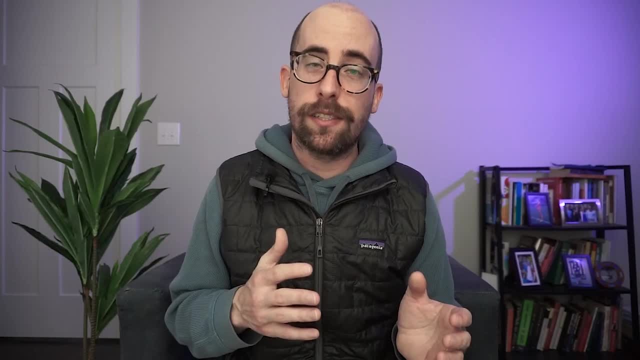 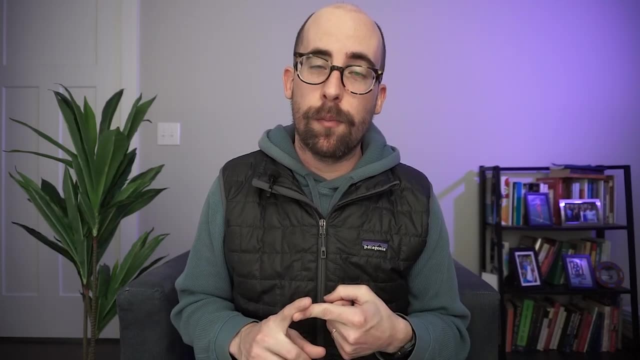 He also has a data product that categorizes product cut launches. that did really well, but the owners aren't working on the product anymore that you could potentially buy. And the point is that number one: data is valuable, People are willing to pay for it. And number two: 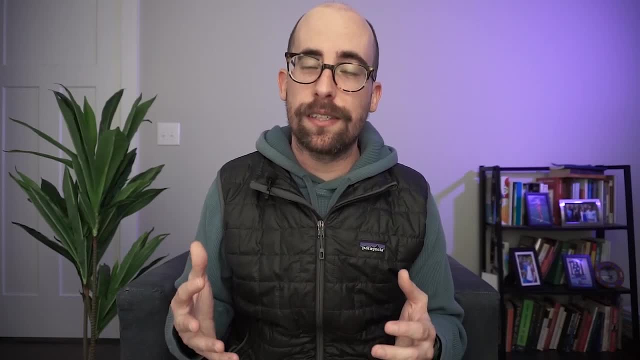 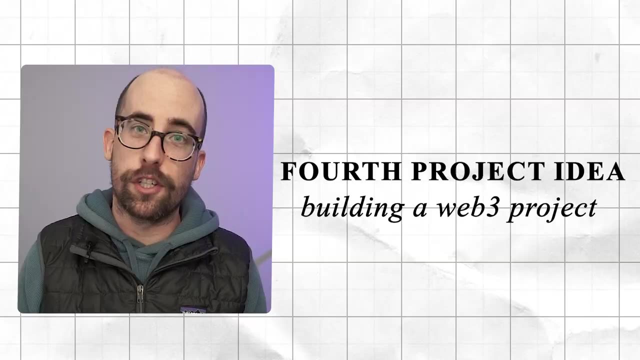 that there's a lot of ways you can go out and get this data, And for those reasons, I think this would make a great portfolio piece. And that brings us to our last project idea, and that is building a web three project. Now, there's a lot of different reasons to build a. 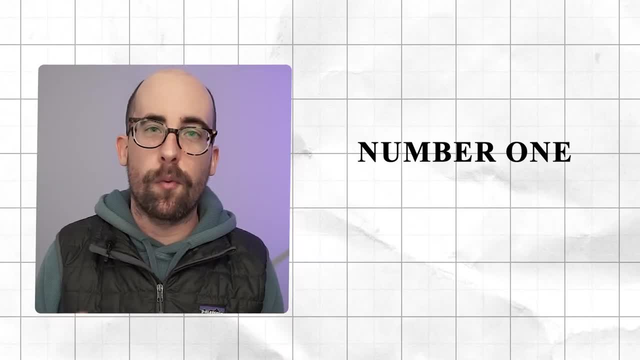 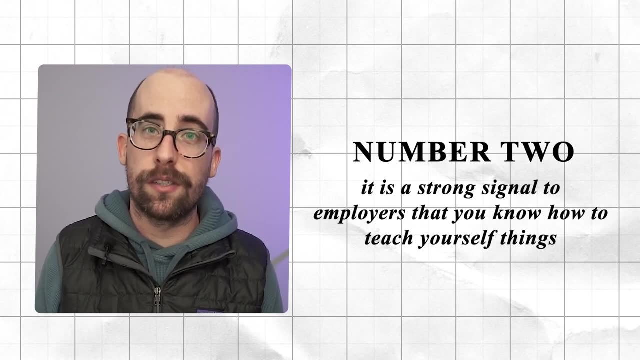 web three project, And it's not just that there's a lot of hype around it. I think number one, this is kind of the next big area. And number two: if you can build a web three project, it's a strong signal to employers that you know how to teach yourself things. 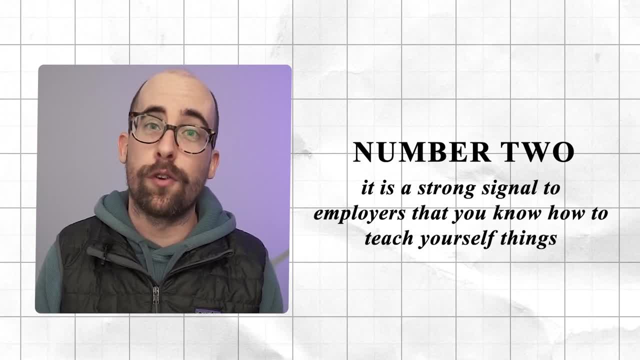 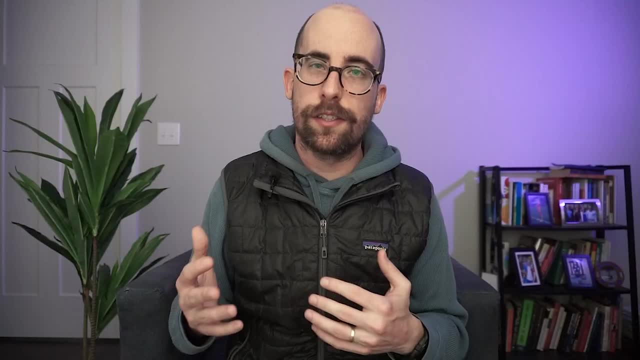 and you know how to learn even when there's not a lot of documentation or tutorials out there. Another reason I think it's very compelling right now to learn web three is that it opens up consulting opportunities. So these skills are in demand, but there's not that many people out. 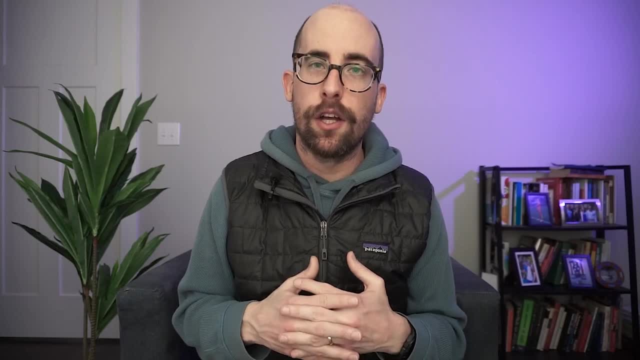 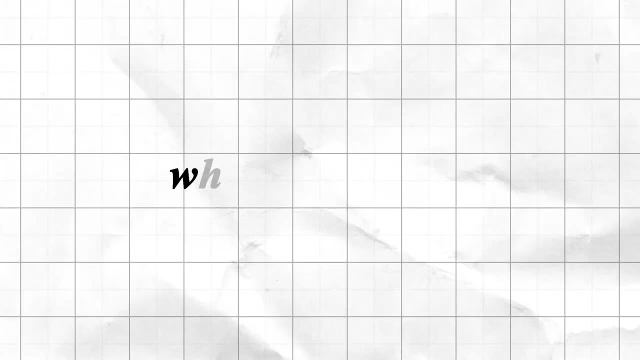 there that know how to build in web three, And so if you have a portfolio piece showing that you know how to do so, you could command some pretty high rates for contracting or consulting work. And so you may be asking yourself: what do I build? 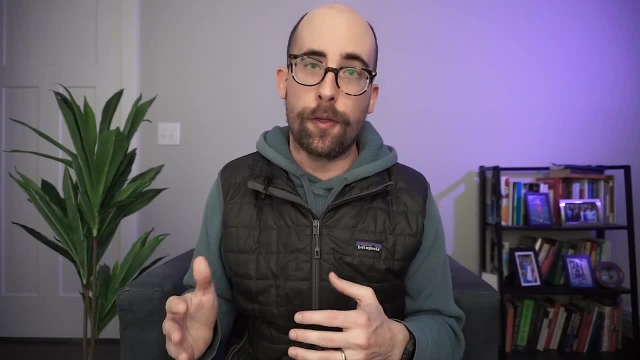 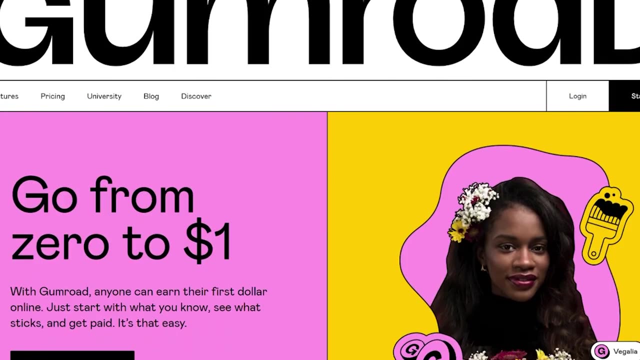 And I think anything that is web two based you could build in web three, especially things that have to do with exchanging money. So you could do a web three version of Airbnb or Gumroad or really anything where you're paying for something You could also. 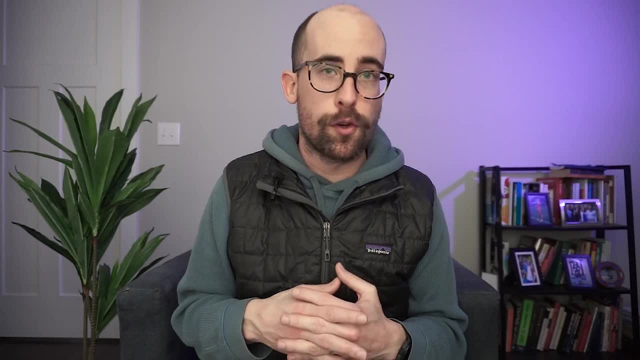 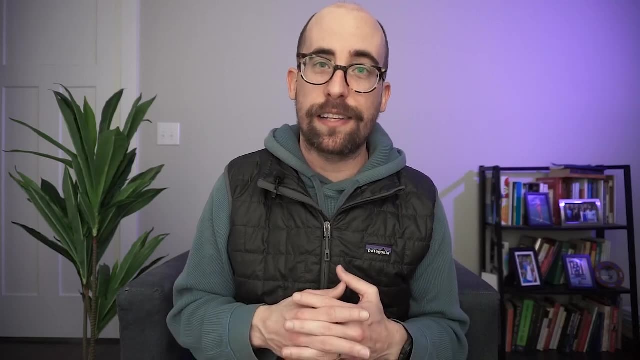 do non-financial things on the blockchain. So I've seen a tutorial example where you have a blog that's built on the blockchain, where that data is stored on chain with its own hash And that's kind of where the blog posts live. So basically, anywhere you have a database. 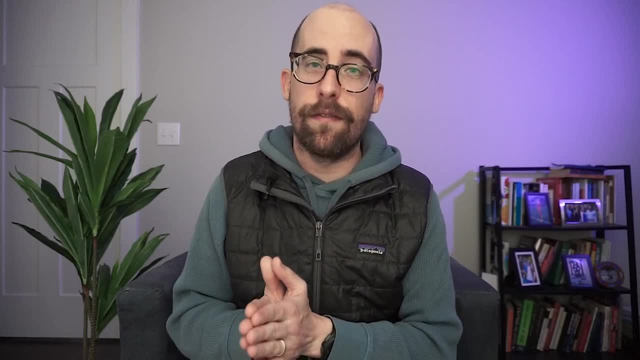 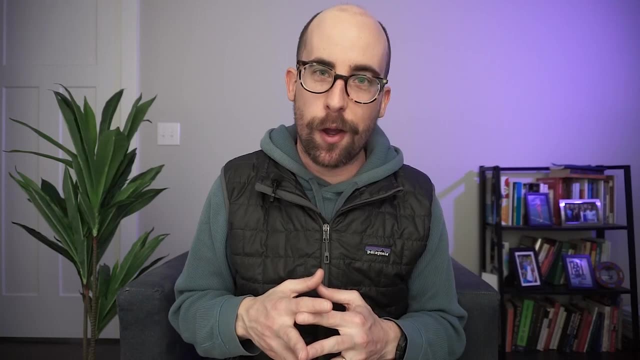 you could sub that out For being stored on chain instead of in some Mongo database that's hosted somewhere, just as an example, And that is actually something I'm working on right now, So I'm trying to take my own advice a little bit, but regardless, I think web three is super compelling. 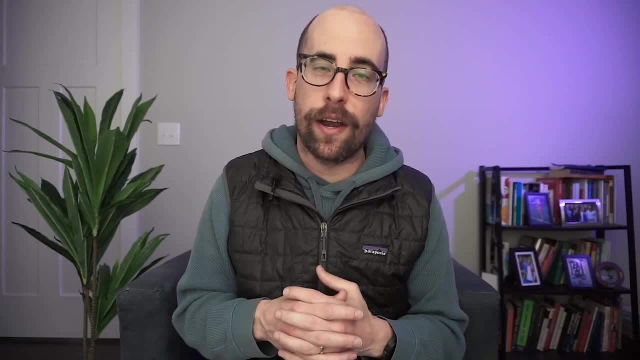 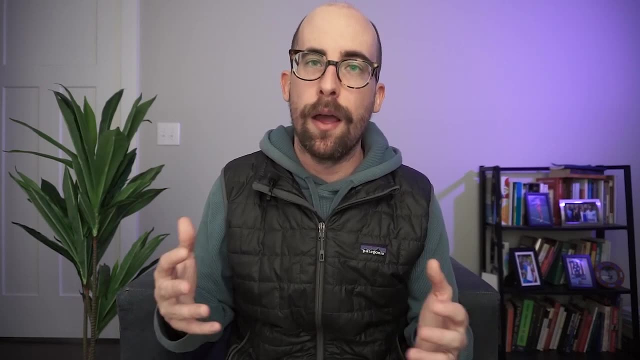 It would make an interesting portfolio piece, especially if you're already in the JavaScript world. I think the transition from JavaScript to web three is simpler because there's a lot of packages on NPM and stuff like that, And so I think it's a great opportunity and something. 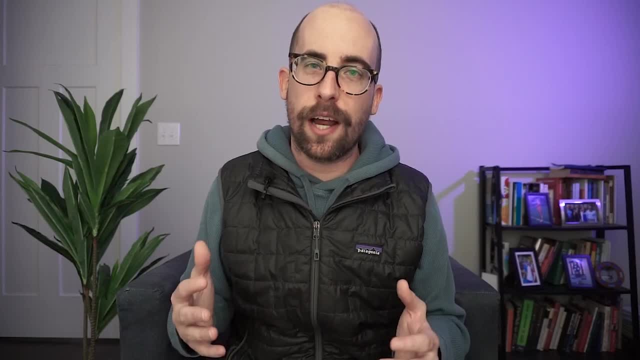 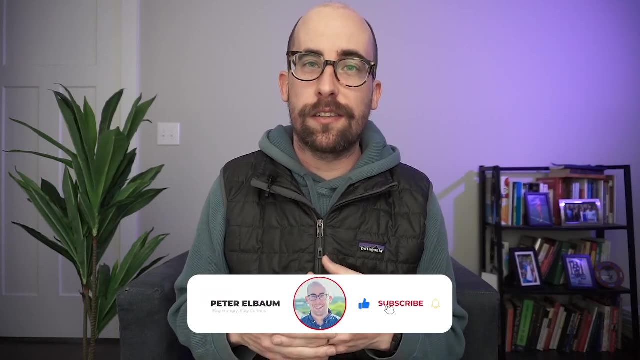 worth considering. Okay, Those are my four best project ideas to get you hired that you could build this week, So go ahead and get started. If you're still here, you'd probably like the rest of my channel, which focuses on software engineering and self-employment, So consider subscribing regardless. Thanks so much.